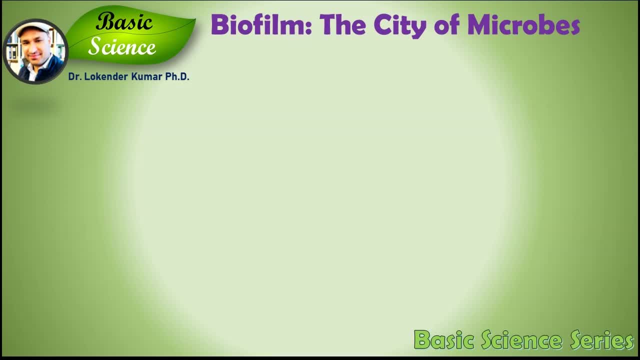 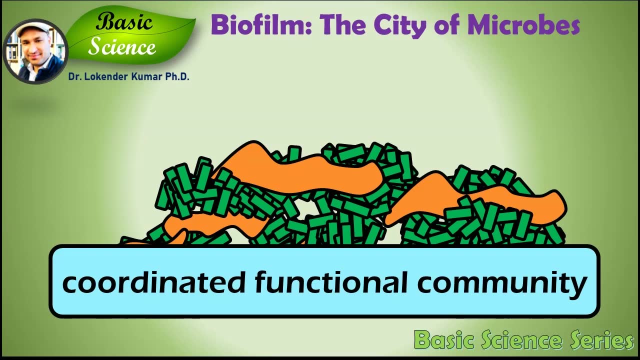 and hospitals In a distance. biofilms look like a hydrogel, but these are more complex than that. These are not just a layer, they are coordinated, functional to create the biomimicry where these bacteria can talk to each other and respond using chemical signal molecules. 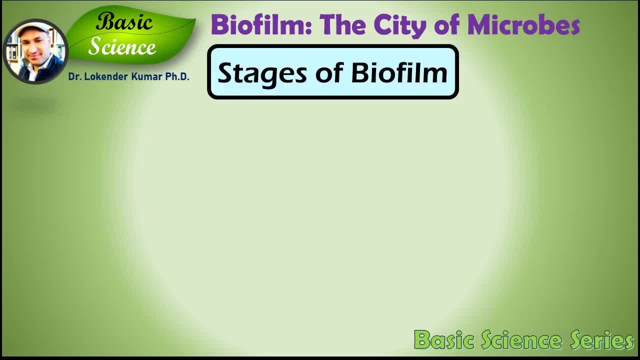 Let's discuss the stages of a biofilm's formation. There are 5 distinct stages of biofilm's formation: Initial Attachment, Irreversible Attachment, Initial Maturation, stage 4, final maturation and stage 5, dispersion. let's start with the stage 1. 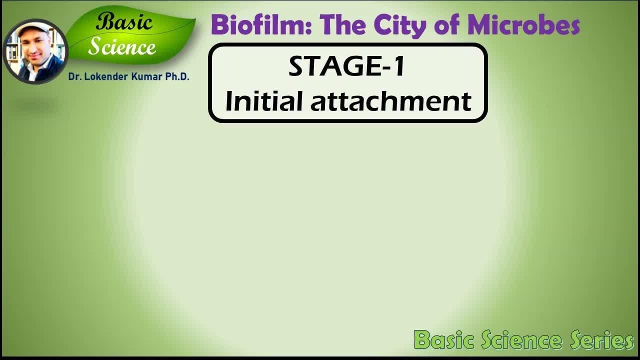 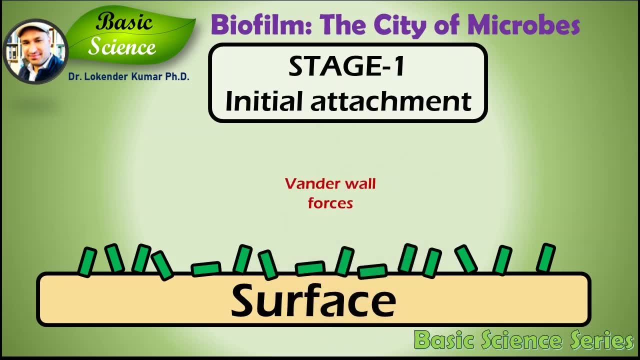 which is initial attachment. this stage starts with the attachment of free floating cells to a solid surface. at first, cell might attach the surface by weak Wonderwall forces. these forces are the physical forces present between molecules and atoms and there is no chemical interaction present. using these forces, bacteria make their initial attachments to a solid surface. 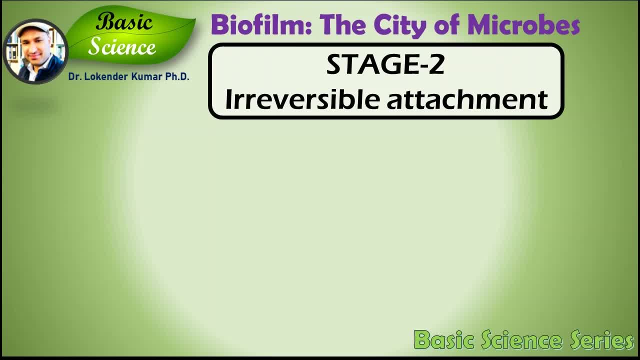 stage 2 is irreversible attachment in this stage if the initial attachment process is successful. bacteria use cell adhesion structures to attach tightly to the surface. most important cell surface structure is pili. pili are the hair like structure found on the surface of many bacteria. another property of bacterial 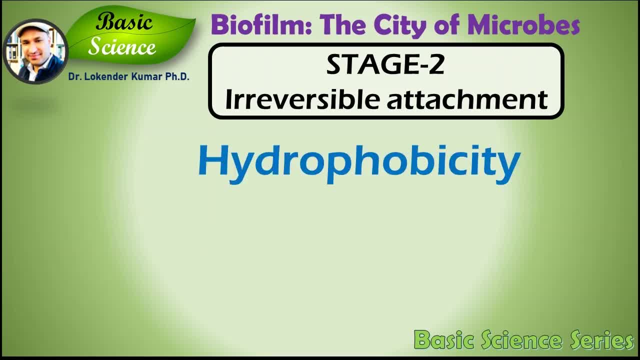 cell. that in the attachment is hydrophobicity. hydrophobicity is the property of molecule that quantify how much a molecule is repelled by the water. most of the time, biofilms are formed in a moist environment, so hydrophobicity helps the cells to get repelled by the water environment and forced to be. 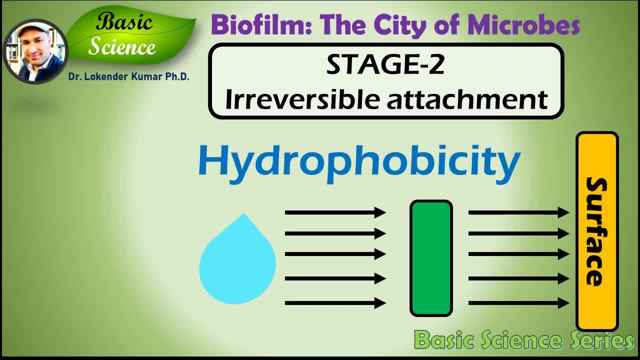 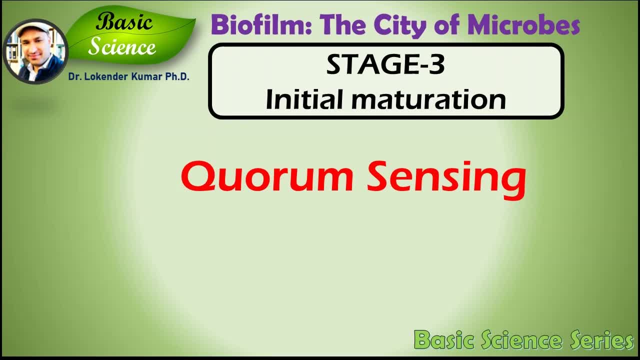 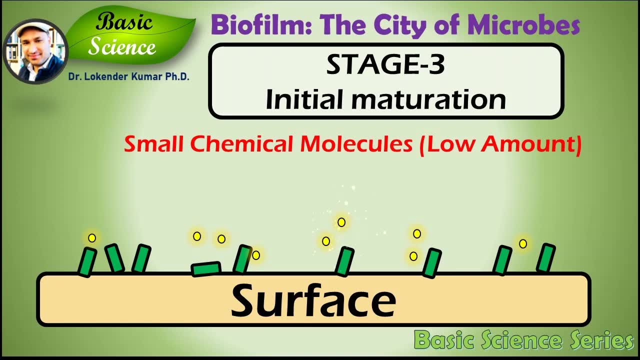 remained close to this solid surface. stage 3 is the initial maturation of biofilm hair cell. communication of the cell with the addition of biofilms is a or. quorum sensing plays a very important role at this stage. microbial cells secrete small chemical signal molecules that are also detected by the same microbial cells. the amount of these molecules 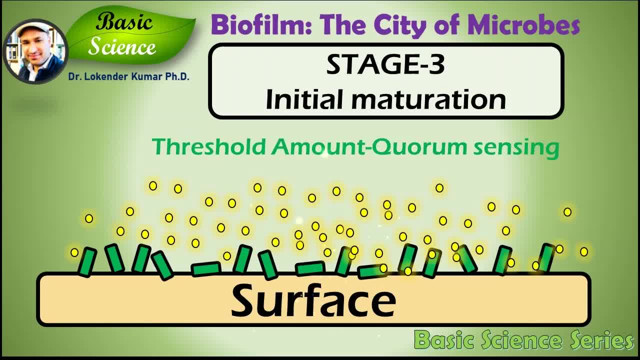 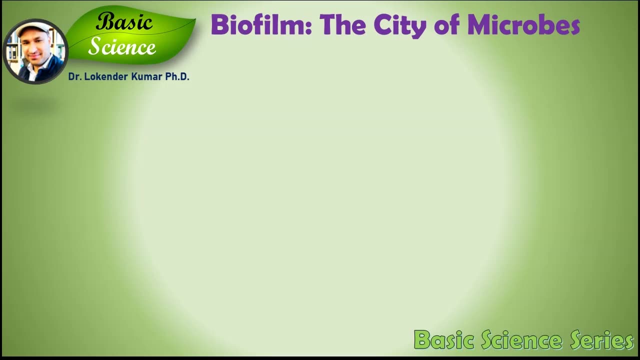 determine the amount of microbial cell present in the surrounding area when the amount of these molecule reach up to a threshold concentration. these molecule induce activation of the cells, and then cells switch the expression of various new proteins. this complete process helps in the formation of biofilm as well as the spread of microbial biofilms. stage 4 is the final maturation. 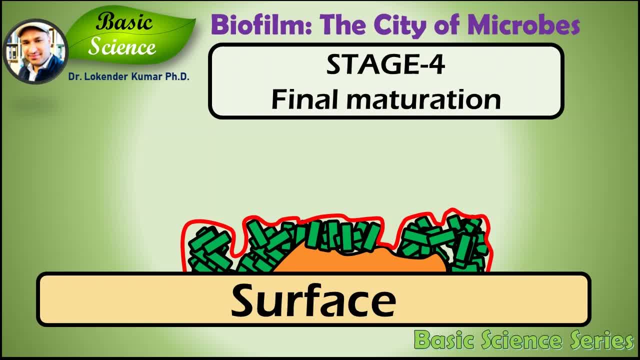 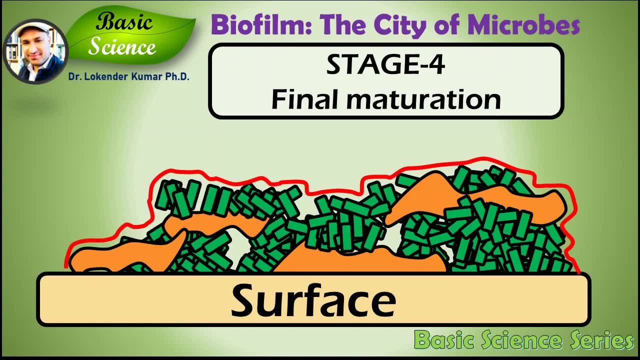 stage. at this stage, bacterial cells start producing very high amount of exopolysaccharide material in their surrounding. this helps the cells to make the huge tower-like structure of the bacterial biofilm. stage 5 is the process of the growth of the bacteria. the cells start producing the 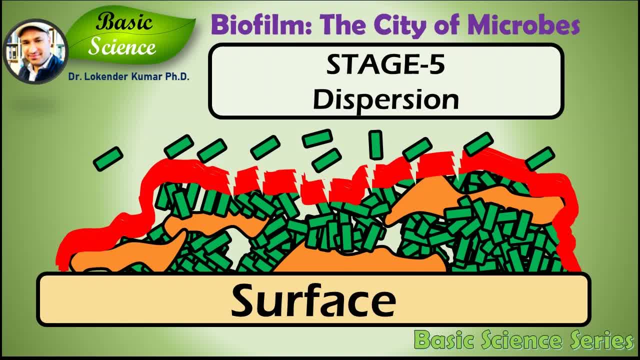 new Всемm différence, and then cells switch the expression of various new proteins. this complete process help dispersion or the detachment stage. at this stage the cells detach themselves from microbial biofilms to look for new area for the formation of new biofilms. if the cell keep themselves to the same. 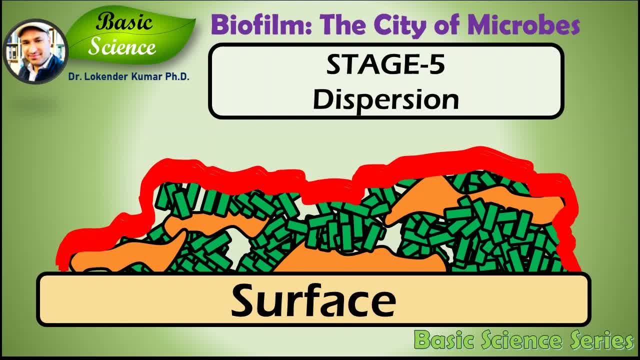 place, the population will grow and the nutrient will be depleted, leading to the death of the biofilm. therefore, for the survival of microbial biofilm, the cell should keep looking for new places to colonize. cells use an enzyme called dispersion b to make their way out from a. 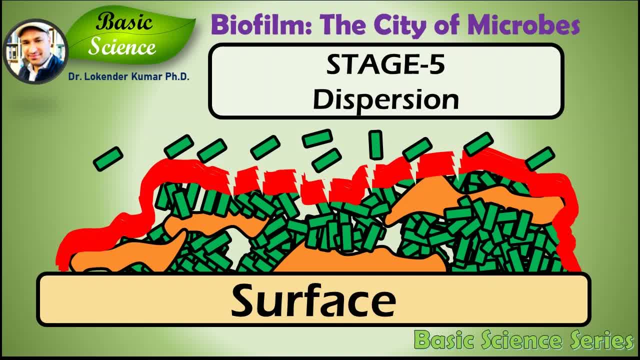 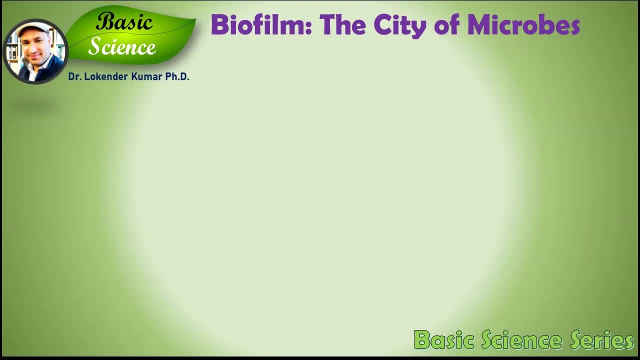 microbial biofilm by degrading extracellular substances. after getting detached from the microbial biofilm, the cells again start with the stage one and the complete process is repeated to make new biofilm. the stage of dispersion fits interestingly to the idea that humans are also trying to find new planets for their survival. we know that is a very important part of our 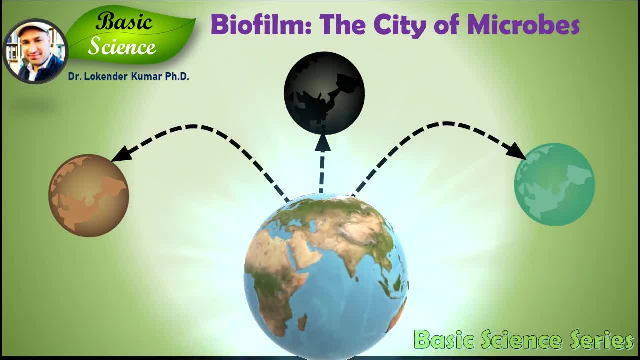 life and we need space food energy. therefore, like microbes, we are at this stage of dispersion to make new habitats so the human community can survive if the resources are finished on planet earth. with this note, i conclude this presentation. please like and share the video with students and. 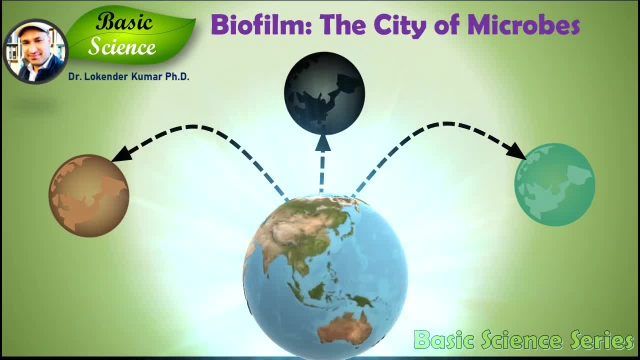 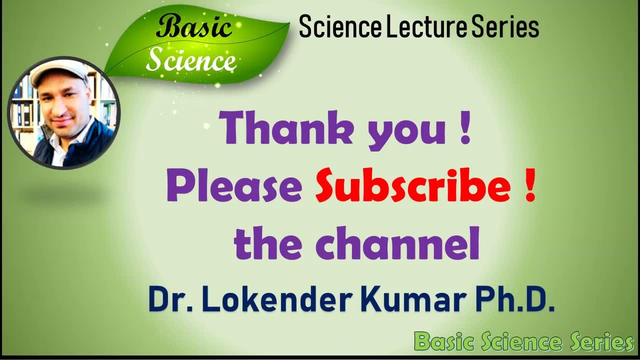 young researchers. please subscribe the youtube channel to get updates on new presentation on basic science topics. please forgive my mistakes. thank you and namaste.